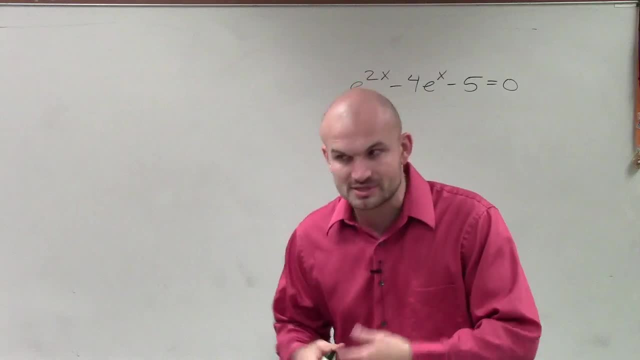 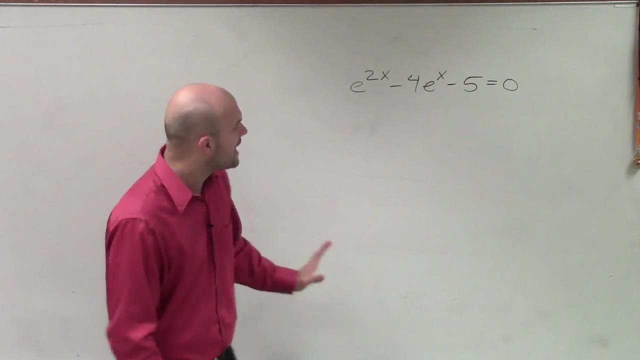 Our common method is isolate the e or take the log of both sides or anything we need to do. This is going to be a little bit different. We see that we have two versions of our e to the x. Now, one thing I look at this is I do kind of notice. 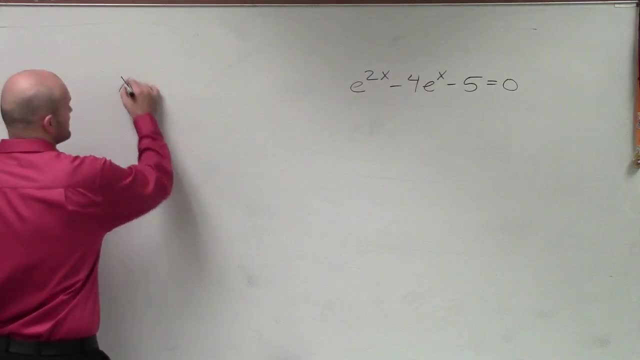 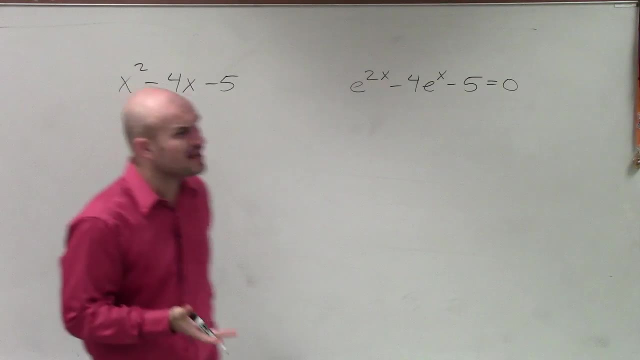 this does kind of look like a little bit of a quadratic, Kind of something like this: x squared minus 4x minus 5. Kind of similar to that. And whenever I get something that looks like something similar to a quadratic, a lot of times I'll do that to say: can I rewrite this? 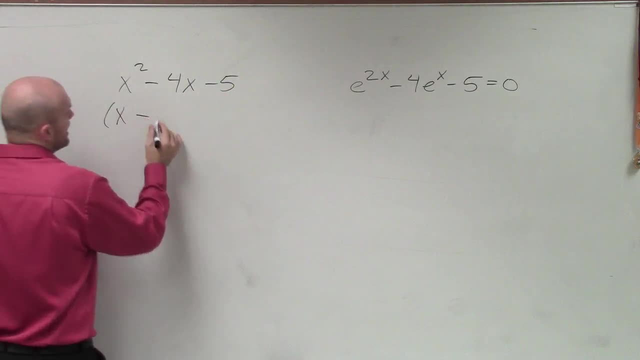 Can I factor this? Well, yeah, you can factor this one. That's going to be x minus 5 times x plus 1.. Right, The factored form of that. Everybody agree with me? OK, So now we've got to see. well, is it even possible then? 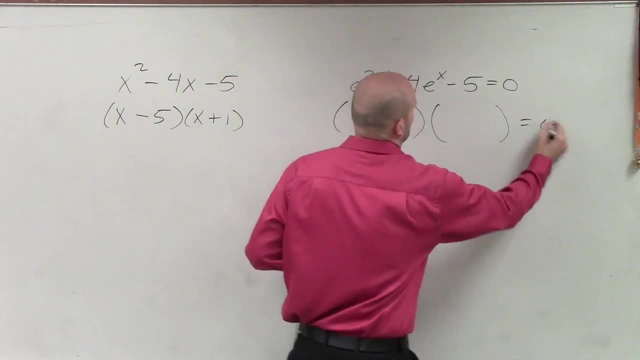 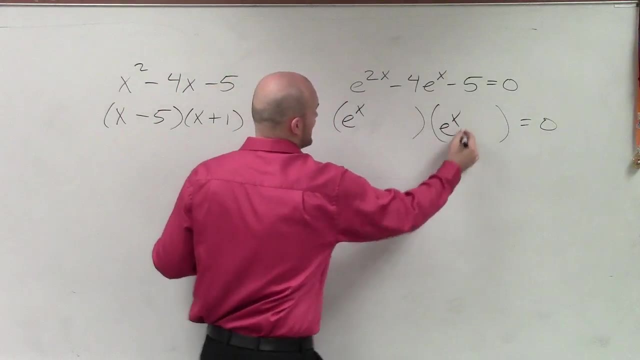 to do that? Is it even possible to do the same thing? So let's go and look at it. What would I have to have- I can't have- if I had e to the x times e to the x? Well, what is e? 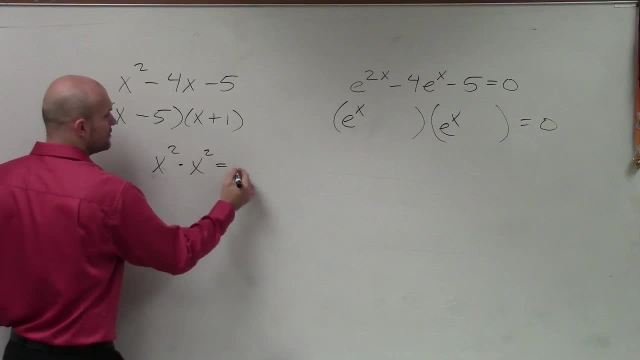 Remember, if I have x squared times x squared, that equals 2x times 2 plus 2.. Right, So if I did e to the x times e to the x, that equals e to the x plus x, which equals e to the 2x. 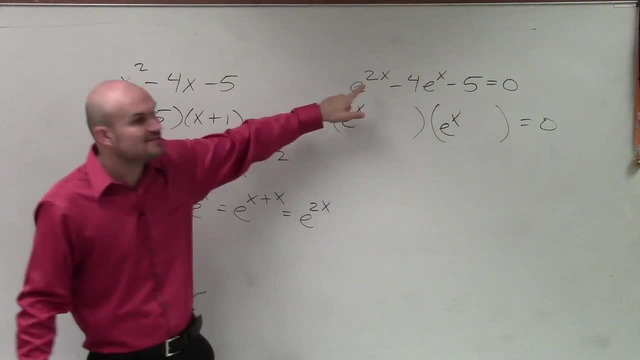 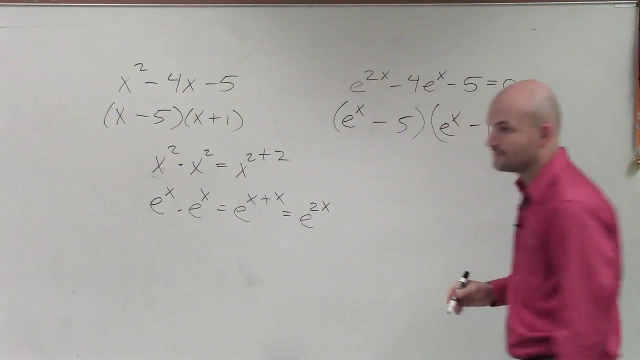 So, yes, actually, multiplying e to the x times e to the x gives me e to the 2x. So therefore, then I can just use these Minus 5,, minus 1.. And if you guys were to multiply these? 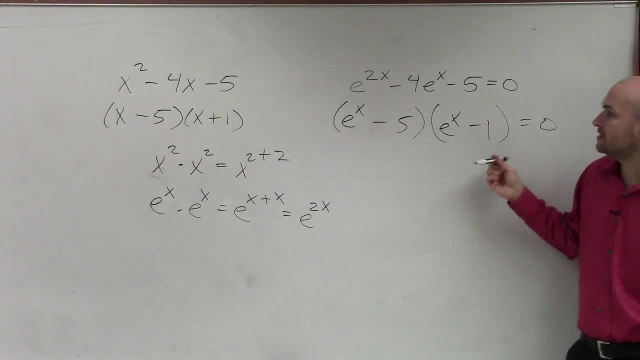 e to the x times. negative 5 is negative 5 e. x. e to the x. oh, that's plus 1,. right e to the x times plus 1 is going to be plus e to the x. Add them up, you get negative 4 e to the x. 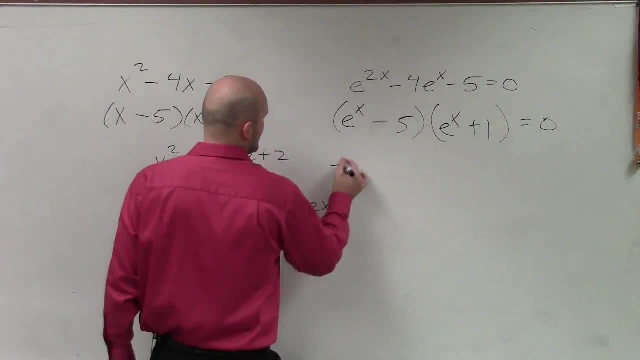 Now I can apply the zero product property, So I can say: e to the x minus 5 equals 0. Right, Yeah, Yeah, Yeah. e to the x plus 1 equals 0.. To solve we write 5, 5.. 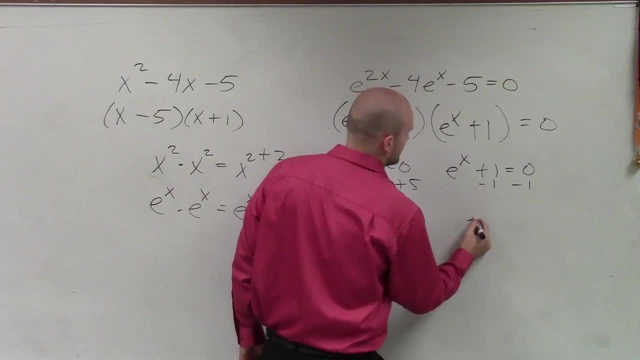 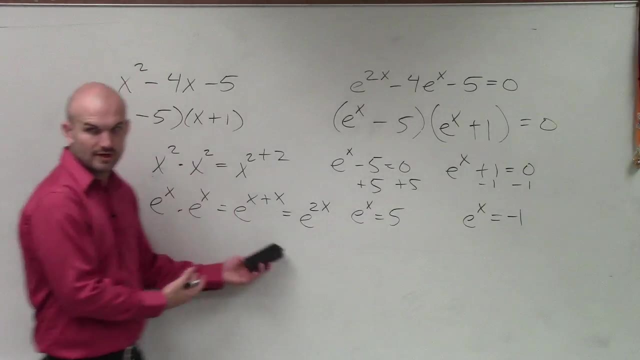 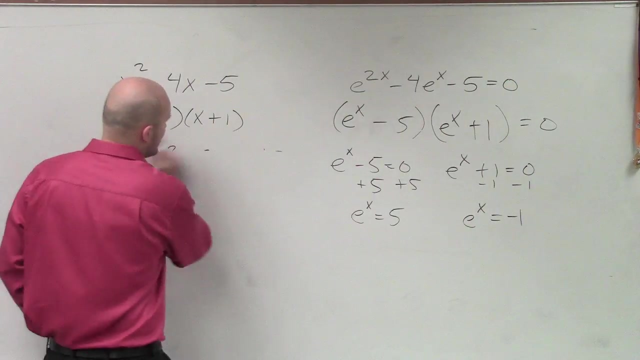 So I say: e to the x equals 5,, e to the x equals negative 1.. Can I erase this over here? So now on our last thing: to go ahead and solve this. remember, we have to solve for x, We have to solve for x.